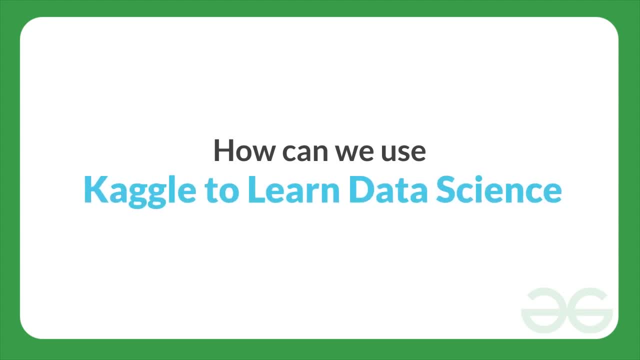 be overwhelming. Finding a community to share a code, data and ideas can seem like overwhelming as well as a far-fetched task, But here's one spot, which is Kaggle, where all these characteristics come together. In this video, we'll be going through in-depth understanding about how can 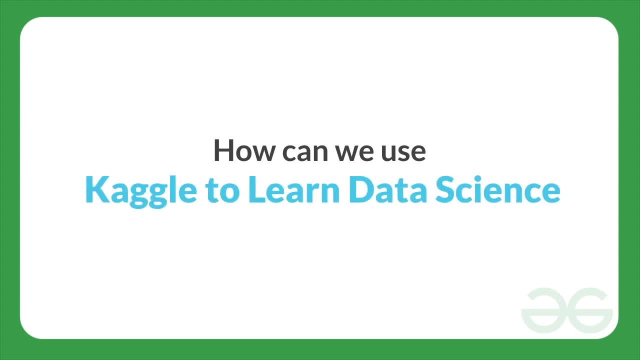 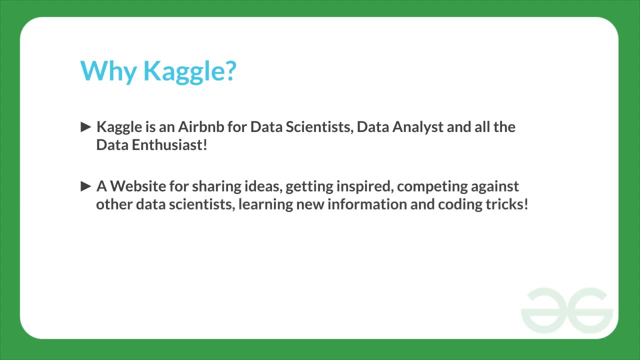 we use Kaggle to learn data science and use that to excel our data science journey. So firstly, let's understand why Kaggle. So Kaggle is an Airbnb for data scientists, data analysts and all the data enthusiasts all over the world, where they spend their days, nights. 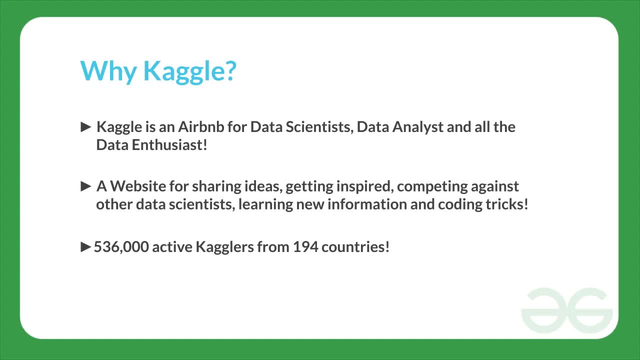 and weekends on it. It's a crowdsourced platform to attract, nurture, train and challenge data scientists, data analysts, from all around the world to solve data science, machine learning and predictive analytics problems. It has over 5,30,000 active members from 1,924 countries and it receives close to, or more than, 1,50,000 submissions. 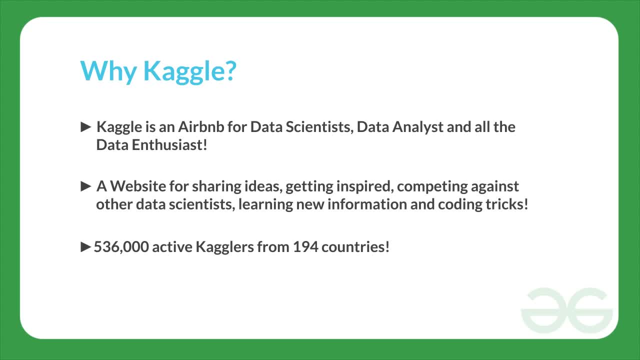 per month. It's a website for sharing ideas, getting inspired, competing against other data scientists or analysts, learning new information and coding tricks, and creating projects, as well as seeing various examples of real-world data science applications. Isn't it amazing? 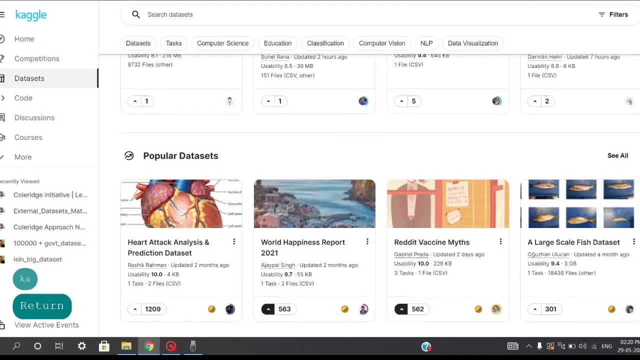 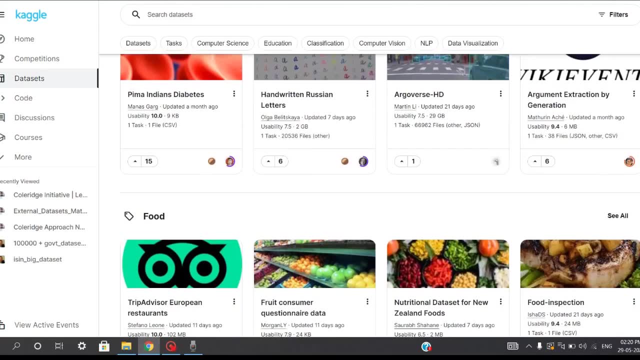 Kaggle is a collection of more than 60,000 publicly available data sets and increasing each and every day by number of contributors all over the world, which can be used for your projects and experiments. With a huge number of data sets available- there are more than. 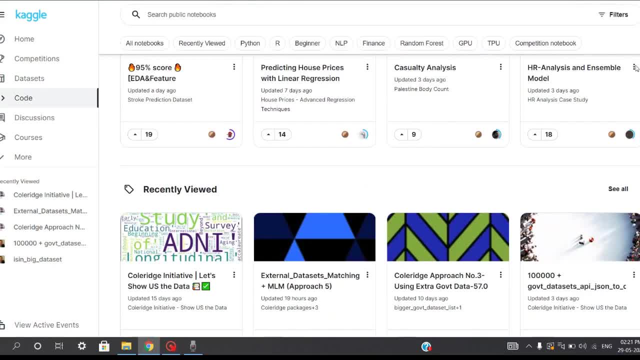 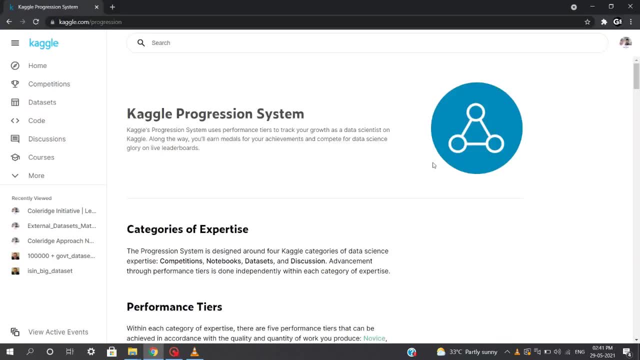 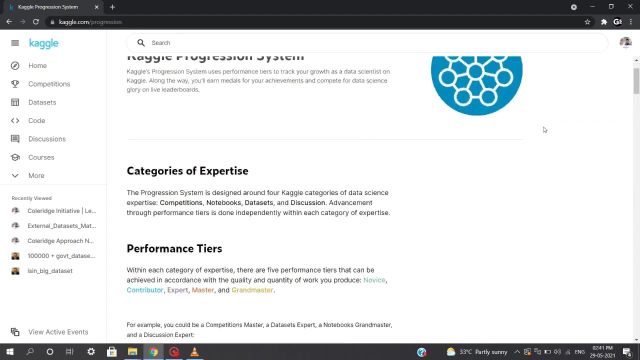 4 lakh notebooks available, which are various different approaches shared by data scientists and analysts on these data sets, which you can learn and collect. Apart from all these, Kaggle also provides an amazing progression system which basically uses performance tiers to track your growth as a data scientist on Kaggle. This system. 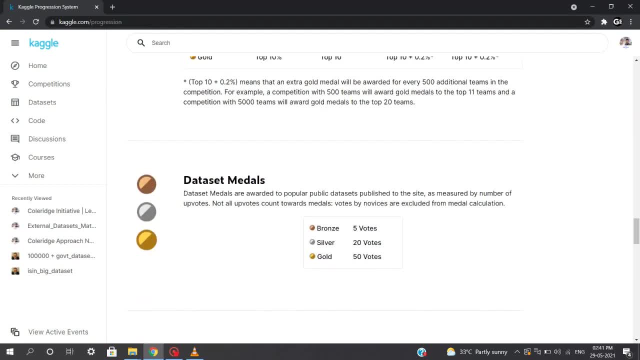 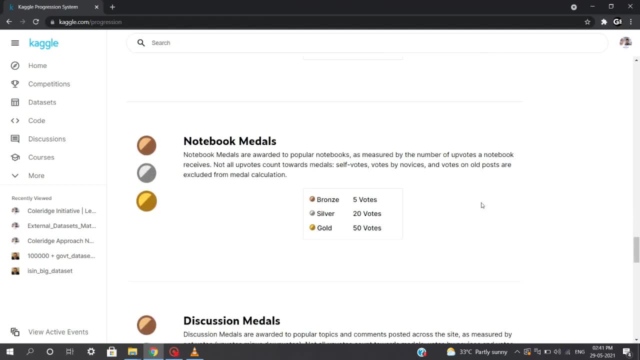 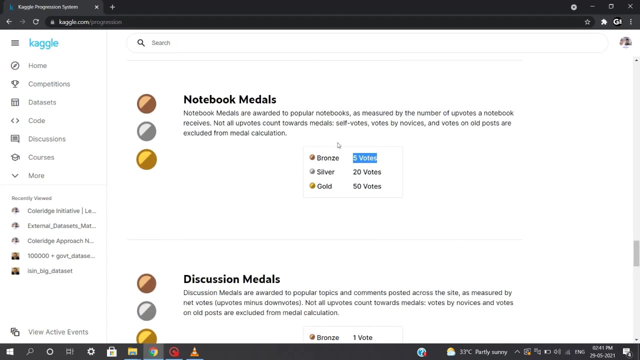 awards and appreciates you for your work done. Each section, such as competitions, data set, notebook and discussions, have a separate progression system which advances you from a novice tier to a grandmaster. one Rules change for each section, like, for example, if you get 5 upvotes. 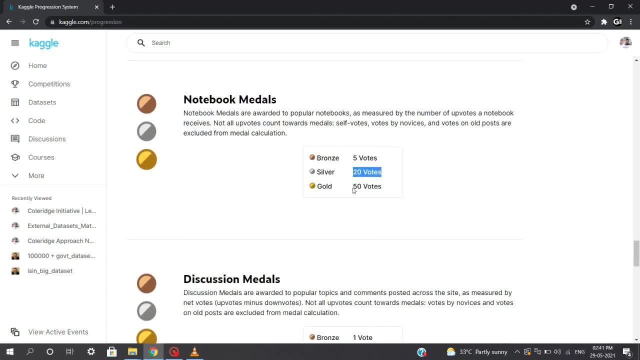 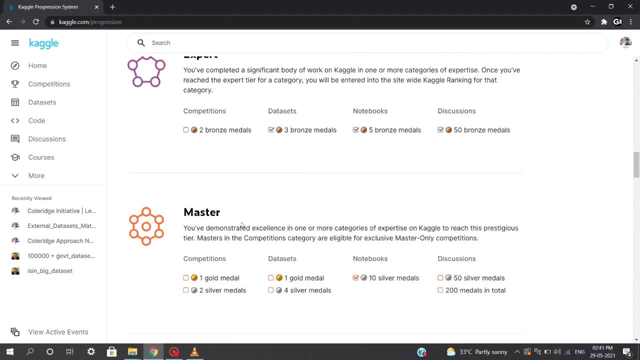 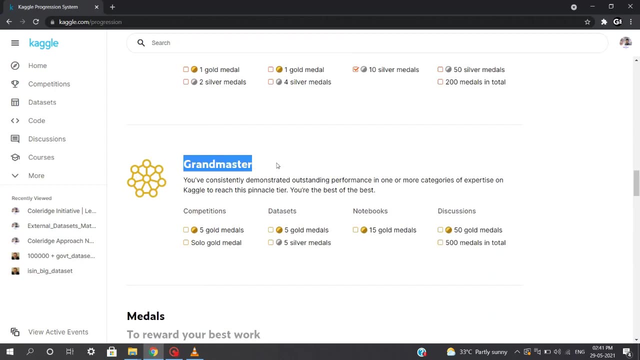 on a contributed notebook or a data set. you get a bronze medal and so on, And as you contribute more and more, your tier increases from a novice to contributor, contributor to expert, expert to grandmaster and finally you reach the most prestigious tier, which is a grandmaster one. 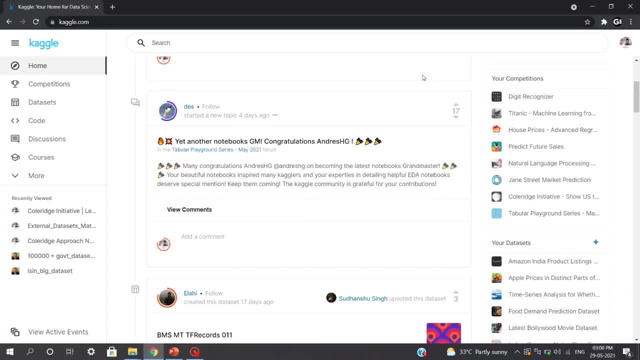 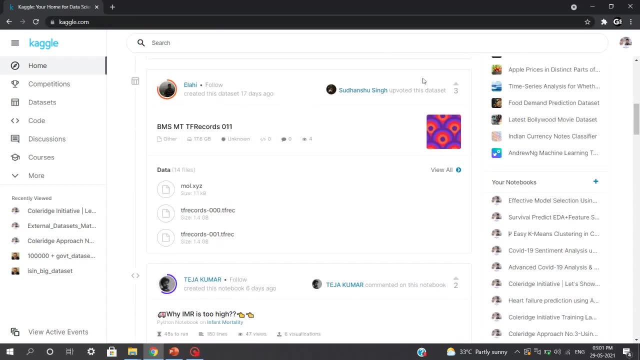 Now let's discuss about each section, such as competitions, notebooks, data sets and discussion sections- in brief, and let's understand how can you learn and contribute on these, as well as what are the performance metrics of each of them. Firstly, coming towards the competitions section, Kaggle competitions are the best. 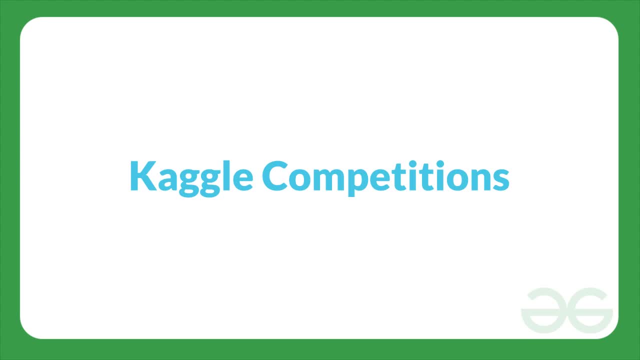 source to test yourself, see how can you rank amongst the peers. Kaggle offers countless competitions, right from very beginner level competitions to advanced level. As a beginner you can always rely on some easier competitions like Titanic survival competitions. You can later try with some recent tabular series competitions as well. 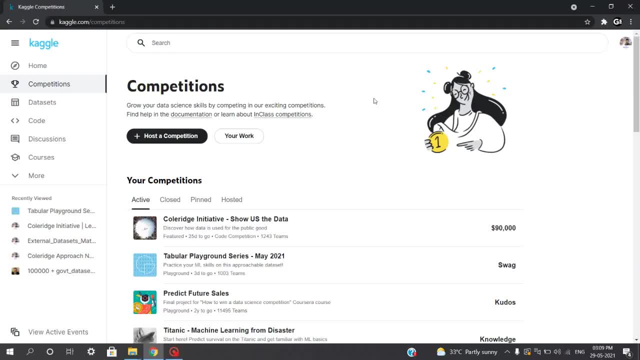 which are organised each month by Kaggle itself. Now let's see how can we deal with the competitions Here. we will be taking tabular series, playground series, competition may 2021, for our example. Now, when you click on the competition, you need to accept some rules and regulations regarding 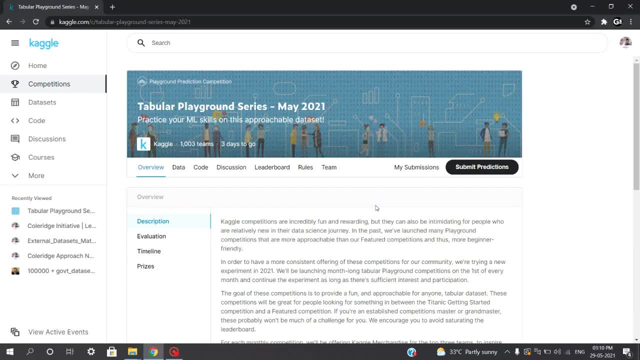 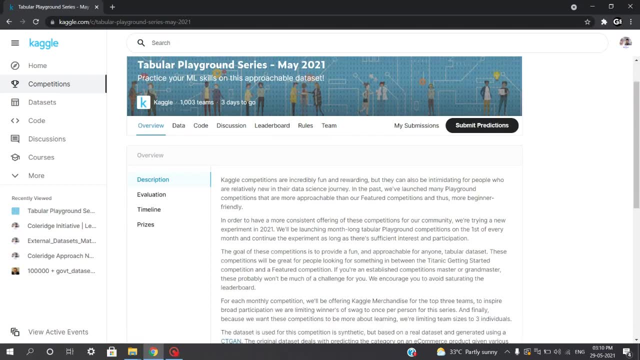 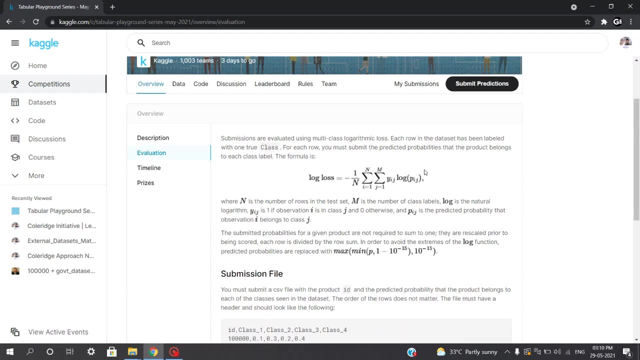 the competition, and this may vary to competition to competition. Now, firstly, when you see, you will be shown with the overview section in which you will get a brief information about what actually the competition is, what are the expectations and etc. Now there will be evaluation section. 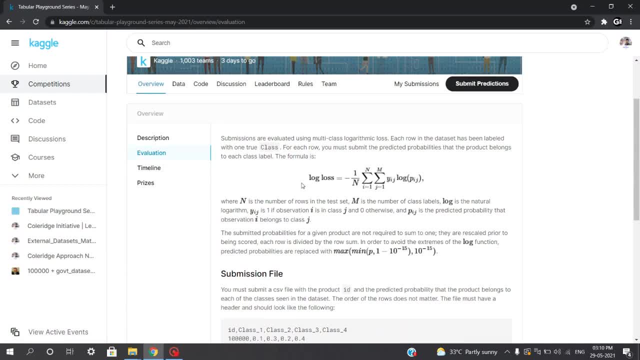 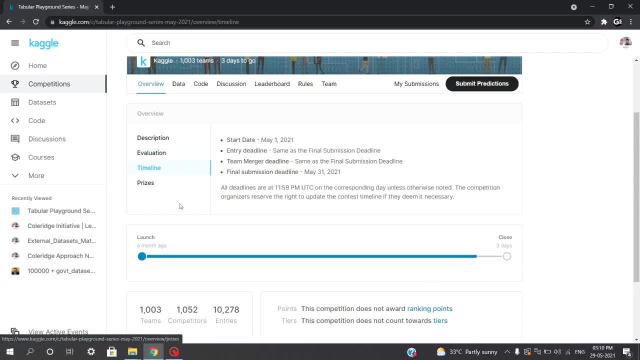 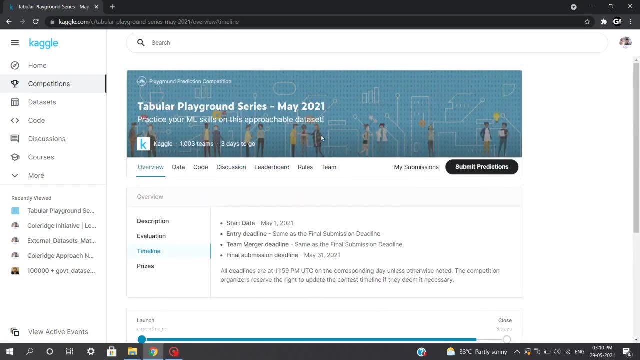 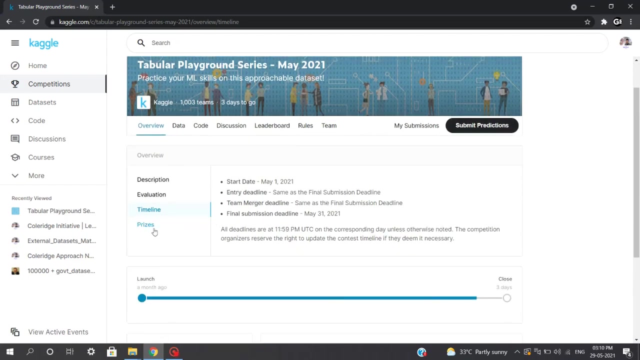 in which the evaluation metrics will be given, what will be considered during your submission and the brief information about the submission file as well. Now there will be timeline, so in some cases, the competition may end for three to four months, while for these particular competition, the playground series one, which are hosted every month, they last for just a month. and finally, the 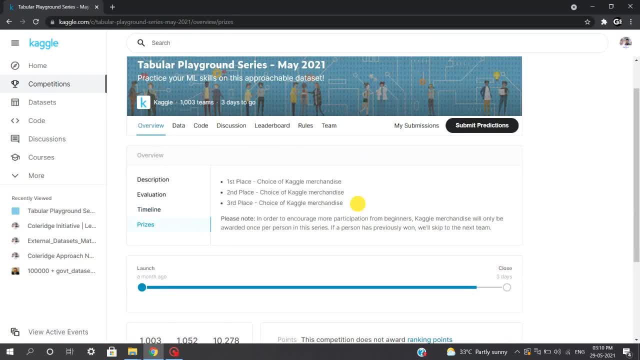 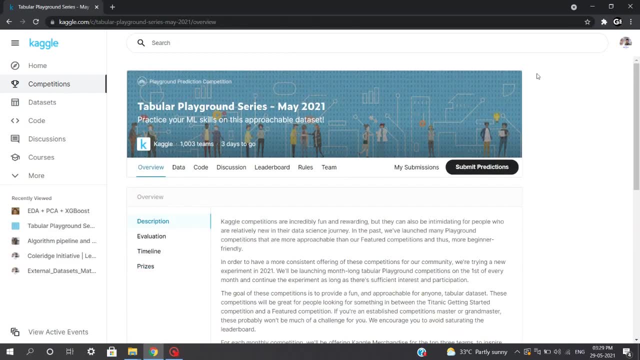 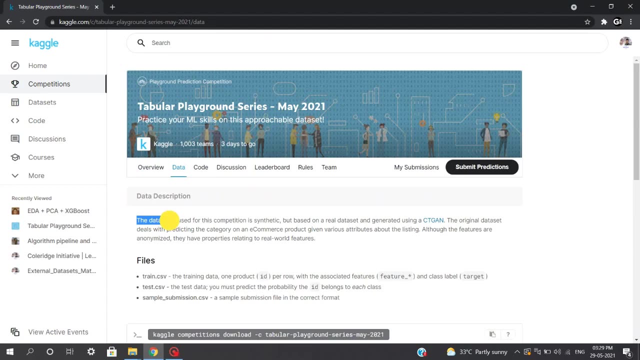 prices. so there are three prizes for this particular competition, But as a beginner, I would suggest that learning should be our first preference than the prices. Once you have got an overview about the whole competition, here is the data section. here you will find the information, a brief information about the data for the competition, and you will 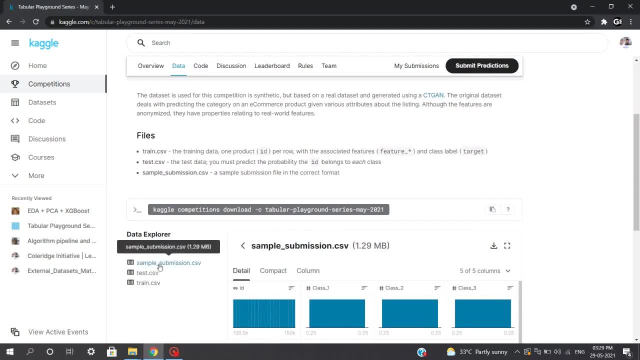 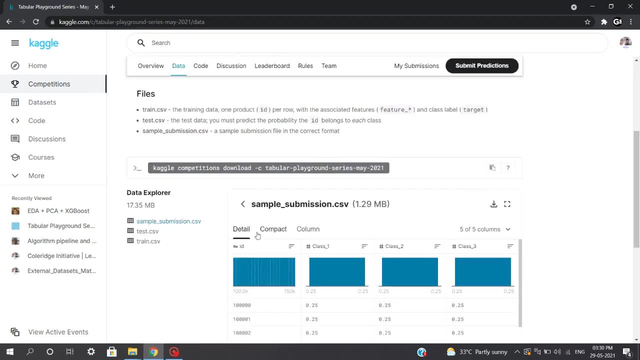 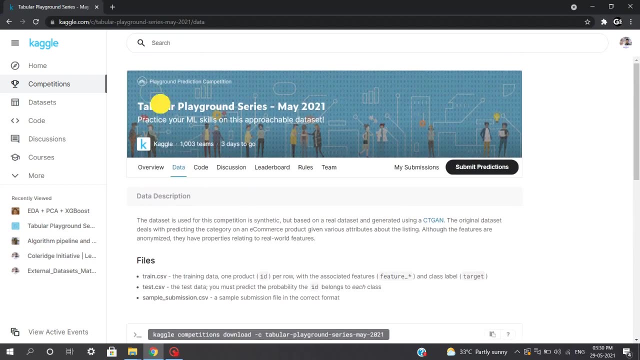 be provided with a train test and sample submissioncsv. so you should train your model using the train csv, you should test the model using test csv and your submission file should look like this. Now, as a beginner, I would surely recommend to go for these tabular series. 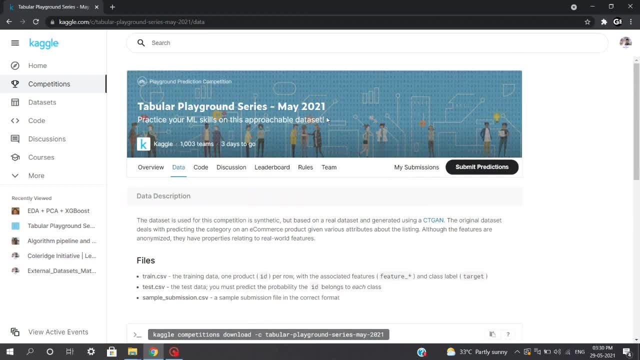 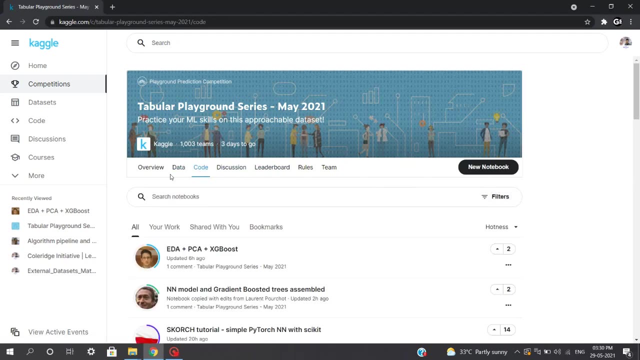 competition which are hosted every month by Kaggle, because these competitions are not very easy. they actually depict the real world scenarios in which you can learn quite a lot of things. Now say, if you deal with this competition and you got stuck somewhere, so the code section is for your rescue. 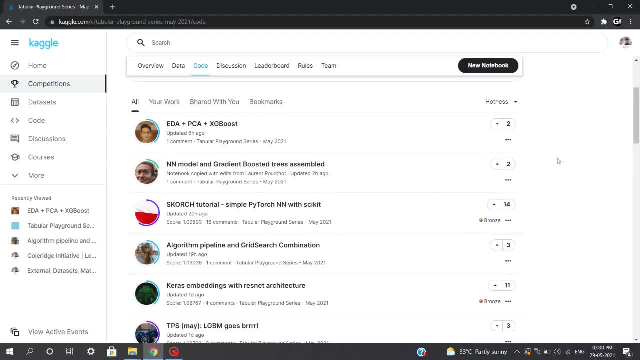 you can find n number of approaches and notebooks. you can find n number of ways to get started by a number of data scientists or analysts all over the world. In the later part of the video we'll be also seeing how can you create your own notebook. 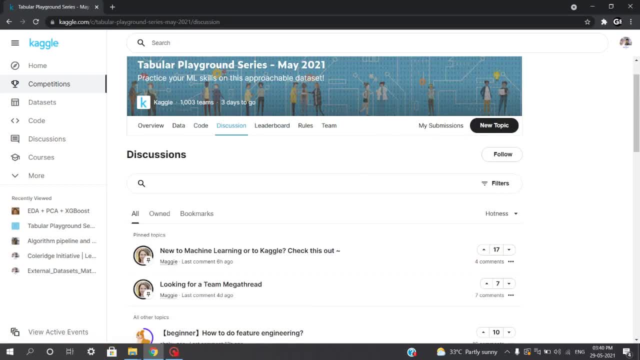 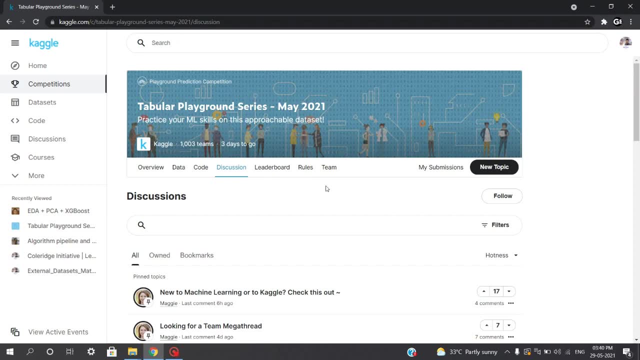 and start dealing with the data set. Now, coming towards the discussion section, say you're dealing with this competition and you find some, find yourself stuck and you don't know some concepts. you can surely ask your doubts over here and you'll be amazed to see that within a day or two. 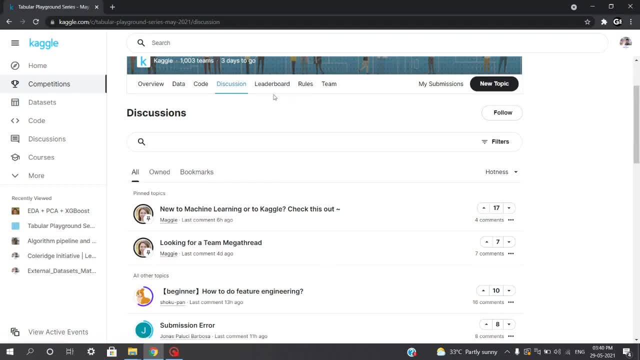 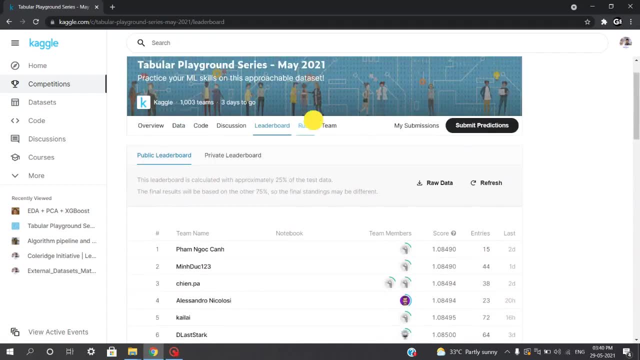 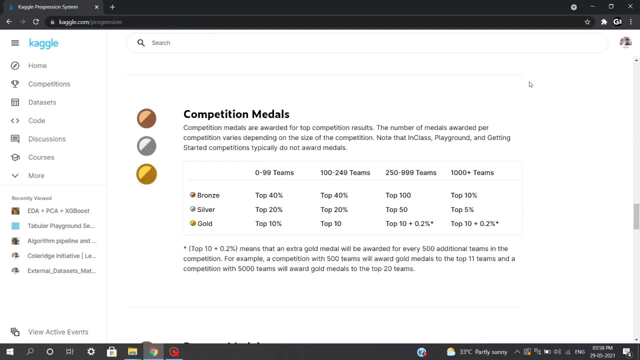 your doubts get solved. Helpful over here. now coming towards the leaderboard. the leaderboard section is where the rankings are displayed and finally, the rules and the team section where you and your friends can participate together. Coming towards the progression of the competitions: the number of medals awarded per competition varies depending on the size of the competition. Say, if you have 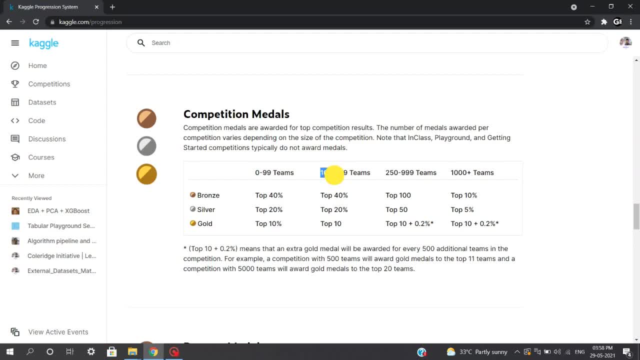 participated in a competition where the participants are between 100 to 249 and you are in the top 40 percent, you will be awarded a bronze medal, or if you are in top 20 percent, you will be awarded as a silver, and if you are in the top 10, you will be awarded a gold medal. 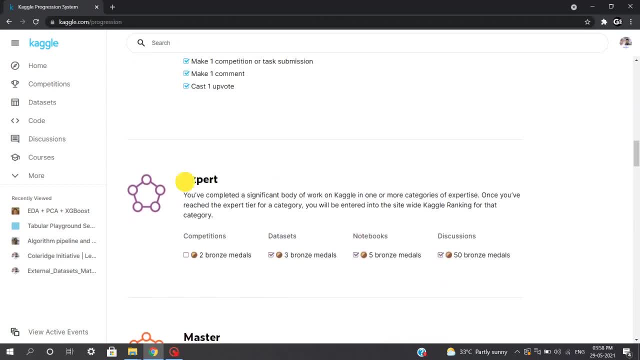 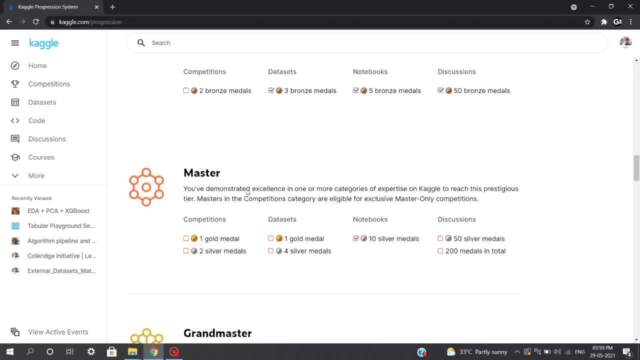 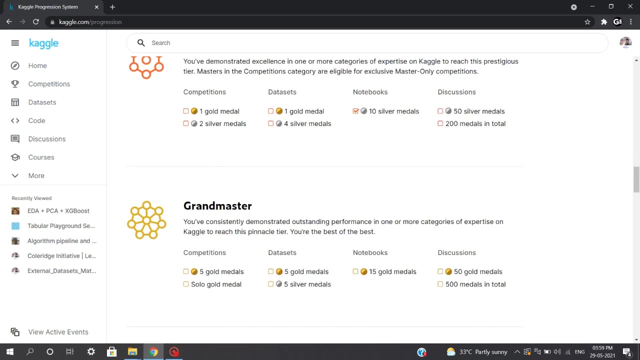 Now coming towards the expert rank. for achieving the expert rank, you should have at least two bronze medals. Now, progressing from expert to master, you need one gold medal and two silver medals. and finally, for grandmaster, you need five gold medals and one solo gold medal, that is, you need to participate as individual. 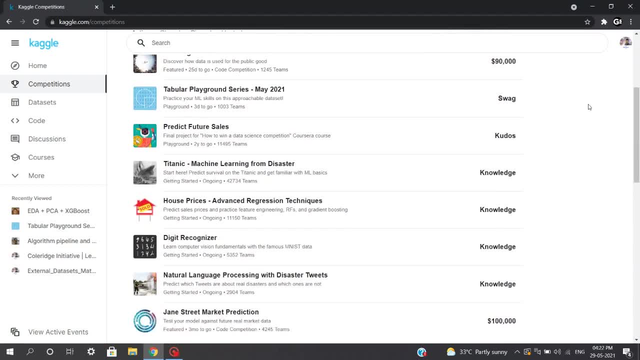 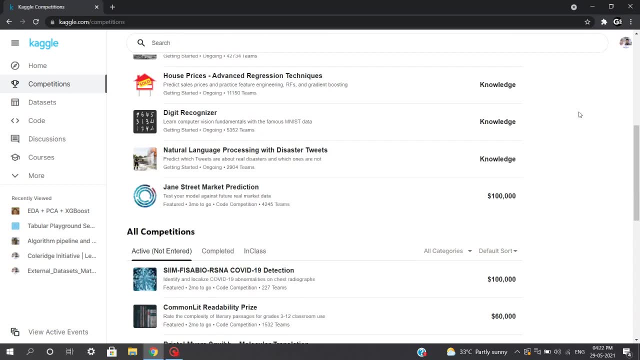 Once you start dealing with the competitions, you get an idea about the real world problems and the scenarios. so trying to decode them surely builds a good data analyst or a scientist within you. If you get stuck somewhere, you can just refer solution by the other cagulars where you 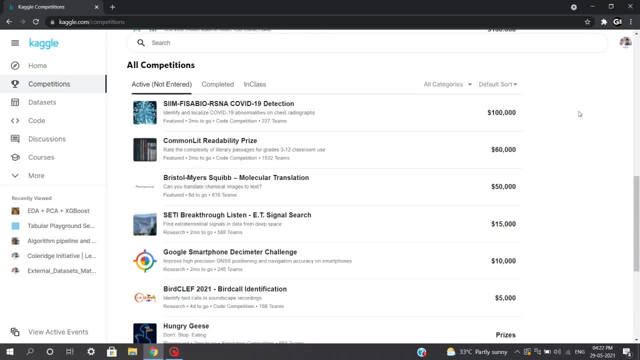 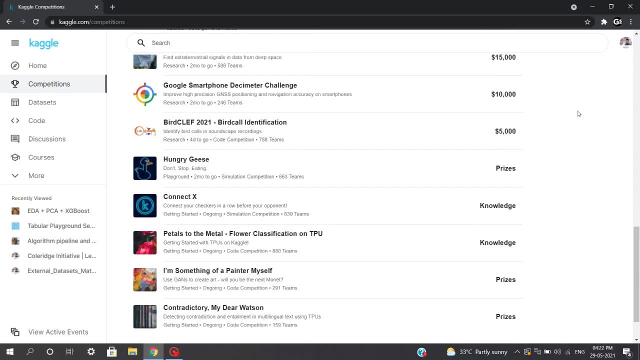 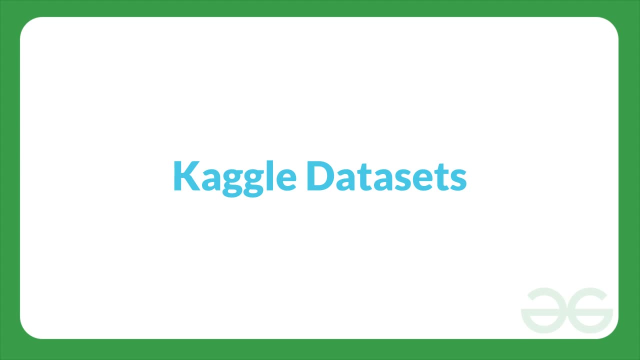 can learn many things: new approaches, new solutions, how a problem can be dealt with- number of ways. This not only improves your knowledge, but also builds a problem solving skills within you. Coming towards the next interesting section, which is data sets. Data sets is not just a simple data. 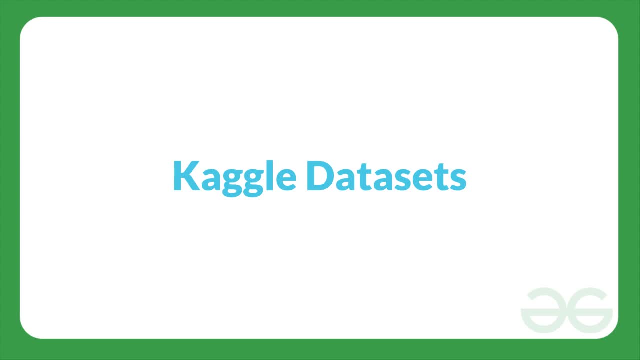 repository. Each data set is a community where you can discuss data, discover public code and techniques and create your own projects. in your notebooks, You can find many different and thousands of interesting data sets of all shapes and sizes. if you can take time to look around and find them, 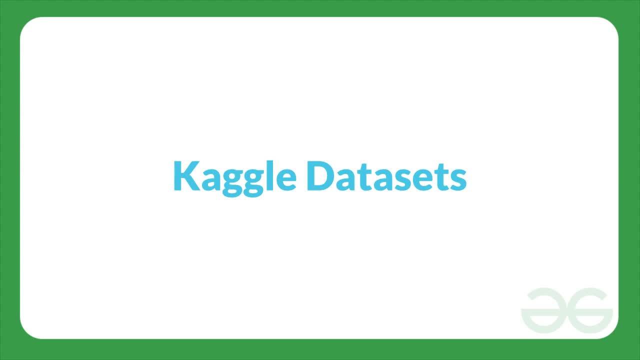 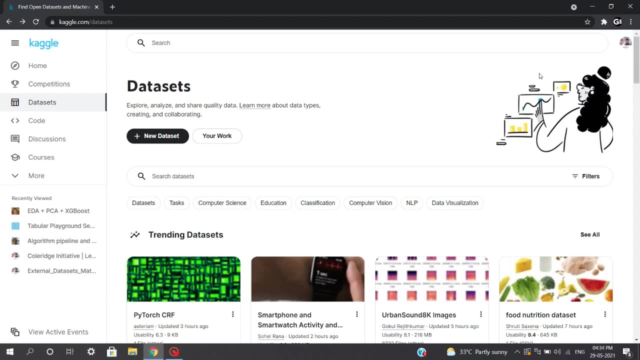 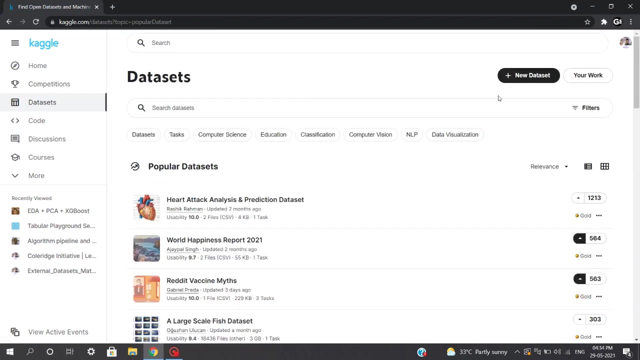 You can explore each data set, explore different approaches, from the notebooks associated with those data sets. also, you can contribute your own data set to the community. There are lakhs of data sets freely available which you can use to enhance and experiment with your data science skills and knowledge. You can choose from variety of data sets with different use cases, just as 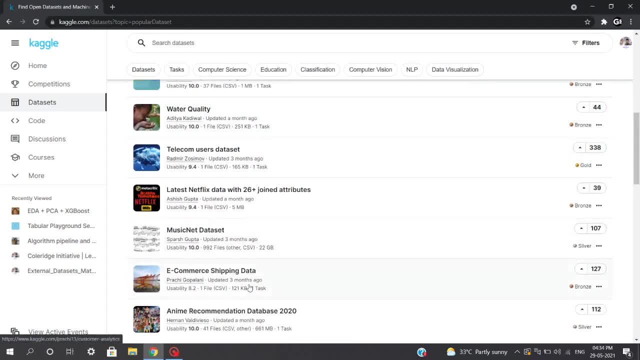 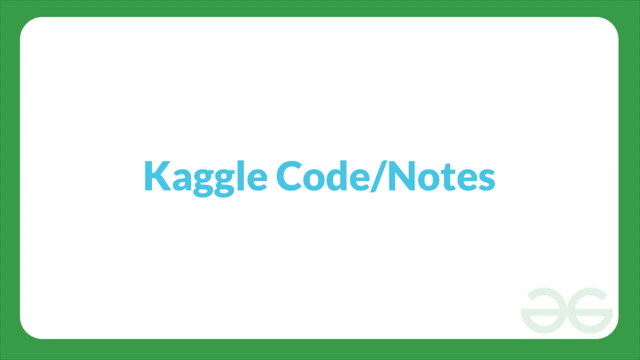 medical, NLP finance and much more for your data science projects. Now let's dive into codes or notebook section. See how can you use the data sets and use them in your notebooks. Codes and notebooks are plentiful on Kaggle. If you want to see countless examples of codes from other Kaggle users, you can easily. 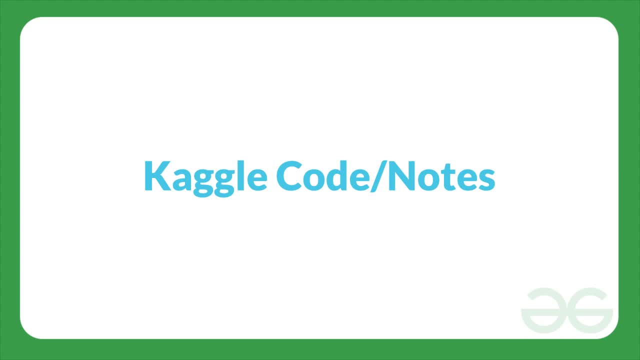 search notebooks that include code as well as the text, where most users comment their code nicely. It's a great way to learn practice and see how others perform similar problems. You can see several examples that will show end-to-end machine learning models. so any problem you ran into. 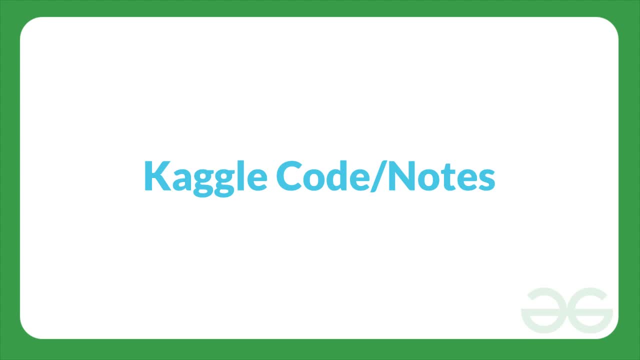 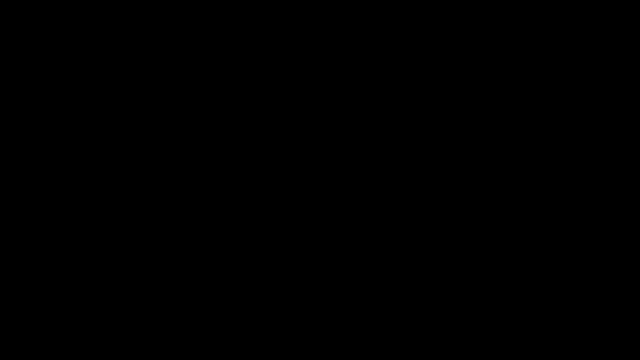 you can search for similar approaches and you'll be amazed to see hundreds of different approaches from which you can learn from. After all, it's about learning and sharing. You learn from other notebooks and share your approaches to the community. Now we'll be seeing how can we use. 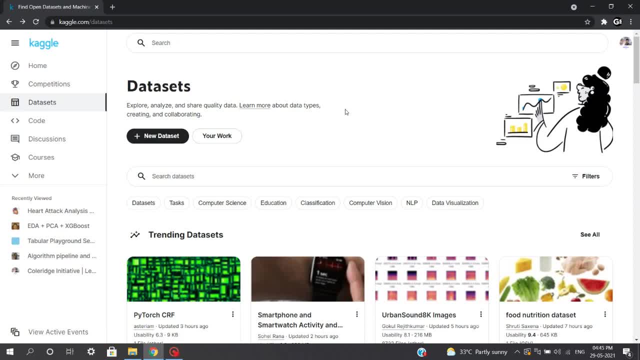 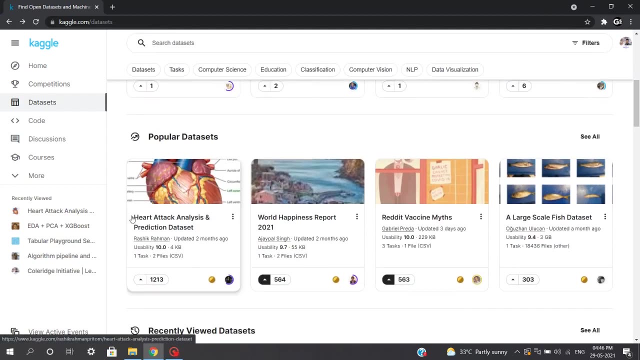 particular data set and how can we create the notebook out of it? and in the notebook, how can we import that particular data set which will be used for our EDA or any machine learning approaches. For that purpose, we'll be using some popular data set: heart attack analysis and prediction data set. 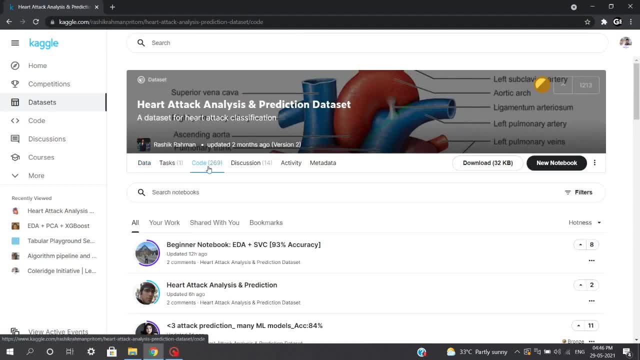 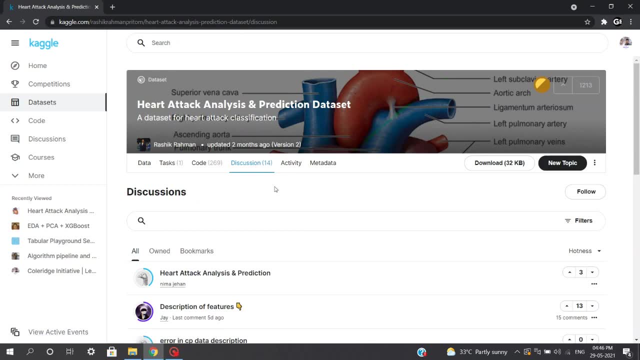 Now, when we click on this, we will find the code where you can see several approaches by different analysts or data scientists and the discussions where people have shared their doubts. Now for dealing the data set, you need to click on the code and the new notebook over here. Now this: 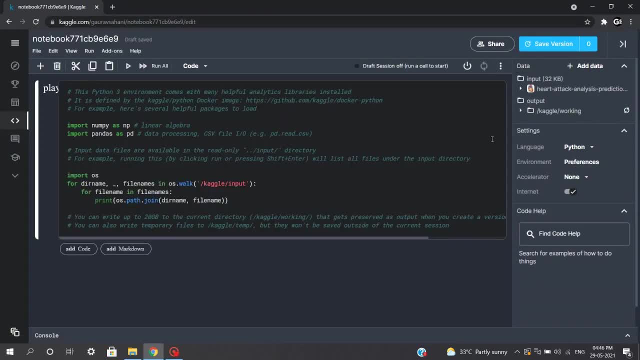 will open up a Kaggle kernel in which, on the right hand side, there will be a input file and the output file, which will be default. The languages: you can select: python or R, the option is yours. The accelerator, so if the task needs a higher computation power, you can also select the GPU or 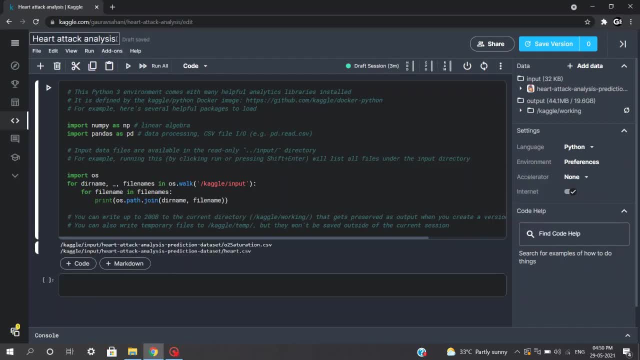 the TPU section. Now, what we'll do is firstly name our notebook as heart attack analysis, for our understanding, and we'll execute the first code, which is the default code, which will import pandas and numpy, As the numbers are already imported. we'll just create a new variable, df, in which we'll import: 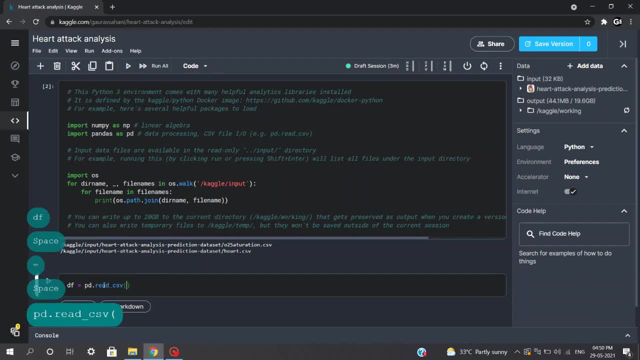 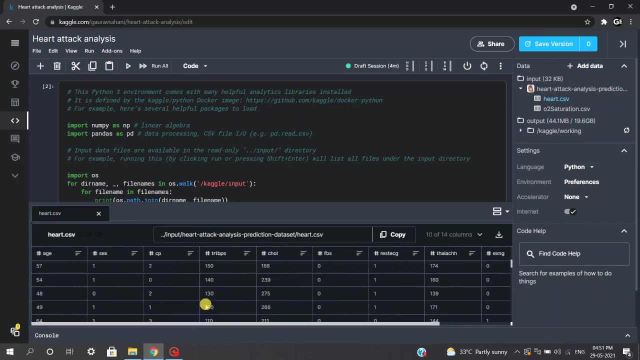 pdreadcsv and we can take the file by clicking over here Now. this will pop up a heartcsv, which is the actual data, and you can see all the features popped up over here Now. just copy the file path from this section and we just need to. 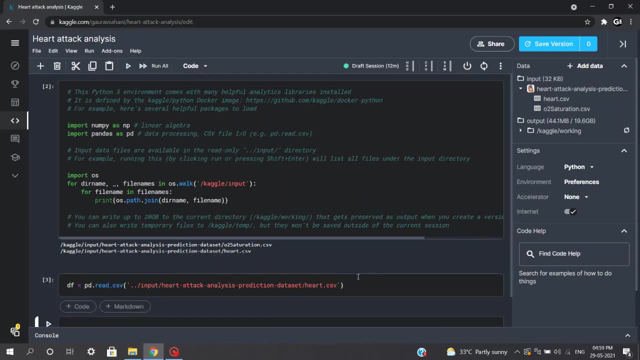 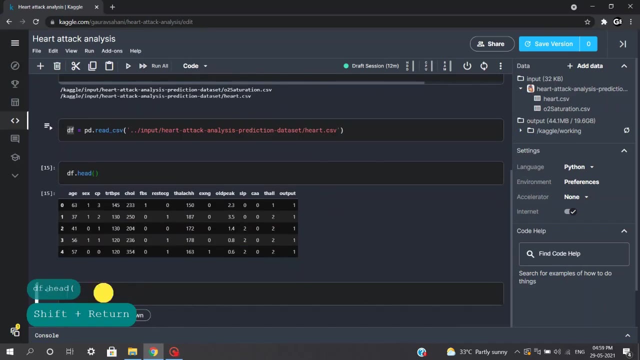 paste this Now. as you can see, our data has been successfully imported using pdreadcsv and saved in our variable, say, df. So let's execute dfhead to see our data and, for the sake of example, we'll just plot a simple histogram of our target variable output. So df output dot hist. 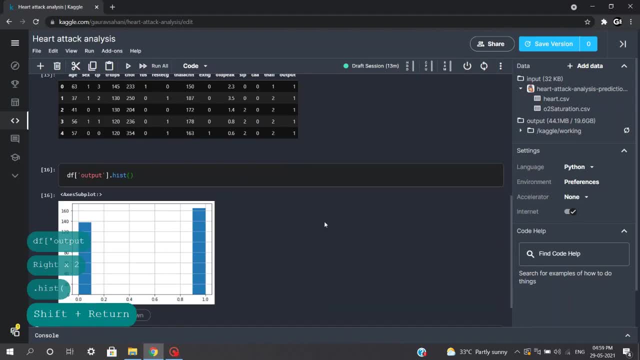 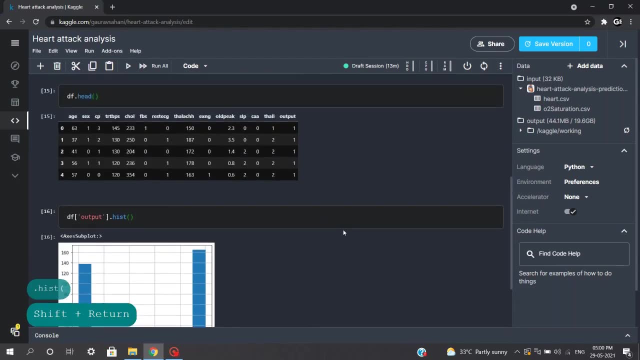 and just like this, we'll plot to see our data And the histogram has been plot. Now, in similar way, you can perform n number of dda, exploratory data analysis, and perform number of analysis on this data. You can create your own machine learning. 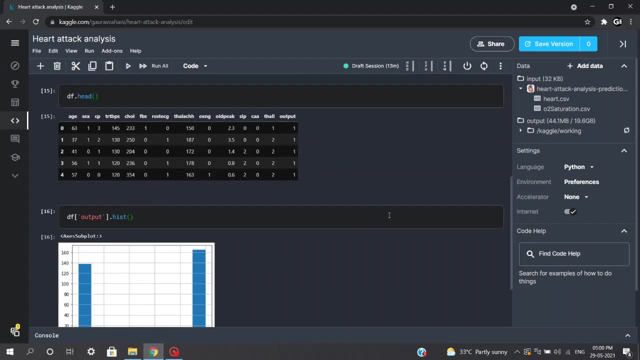 models, experiment with the data and experiment with your skills. If you need more computation, you can just choose accelerator as GPU or TPU. it depends upon you to share that notebook with the community or keep it private. so if you wish to share your amazing notebook with the community, you 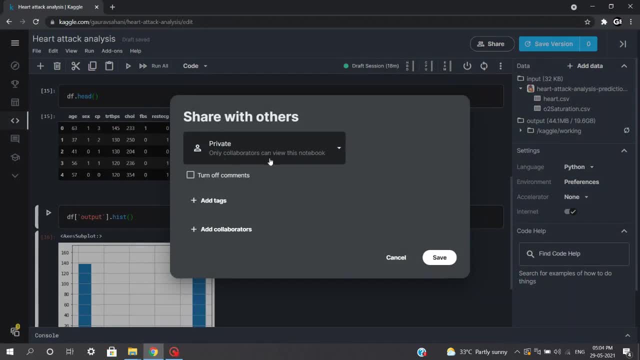 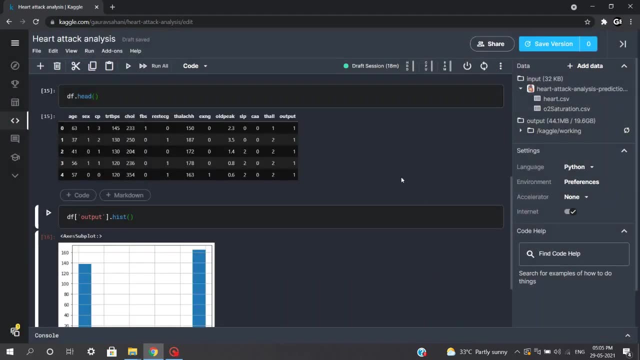 just need to click on the share option. by default, it will be private. you need to click on this and click on public and click on save now. automatically, when you click on save version, your notebook will be shared with the community. now let's click on save version. you can name this version as anything, say v1, which. 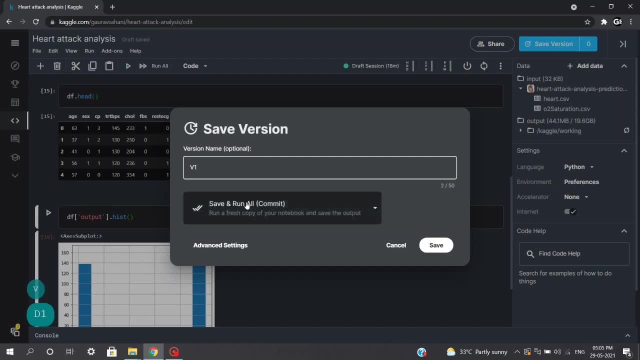 represent the version one and there are two option in which you can choose from, that is, save and run all and quick save. so quick save will save a version of your notebook the way it currently looks, and save and run version will run a fresh copy of your notebook and save the output. so here will be just executing. 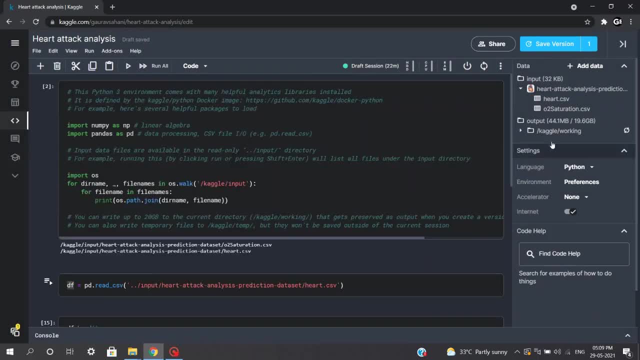 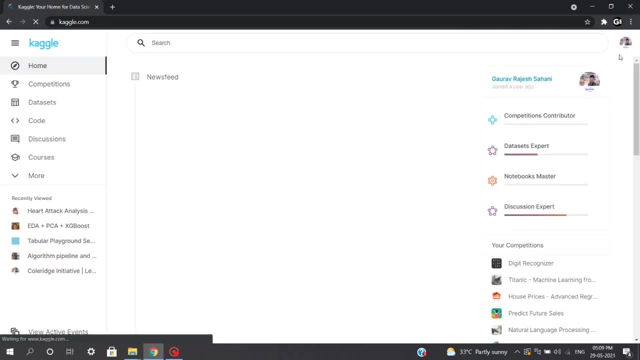 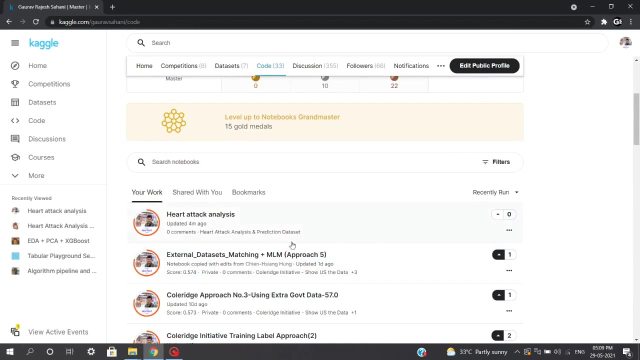 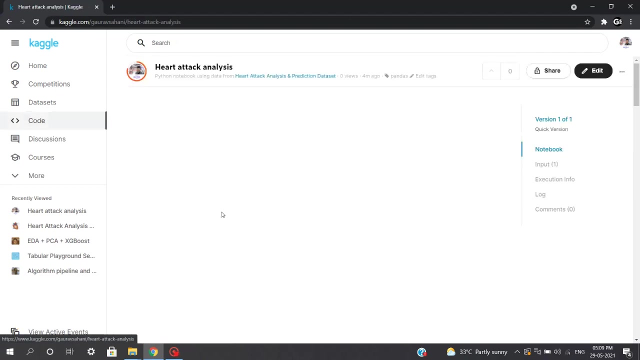 quick save and save now. as you can see, the first version of our notebook has been saved successfully and when we click on our profile, say this is my profile and in the core section you can find my new notebook, published openly with the community. so anyone who wish to see my notebook and watch my notebook and they can have an. 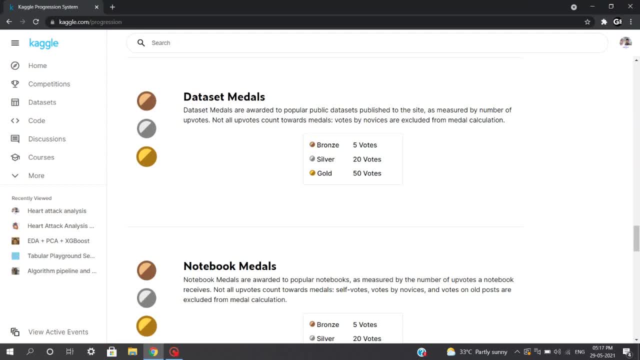 even upload this talking about the progression, the progression rules for the notebook and how to make your notebook better, and that's why i am going to show you the process of how to make your notebook better and more efficient, and if you are getting five upvotes, you will be awarded with a bronze. 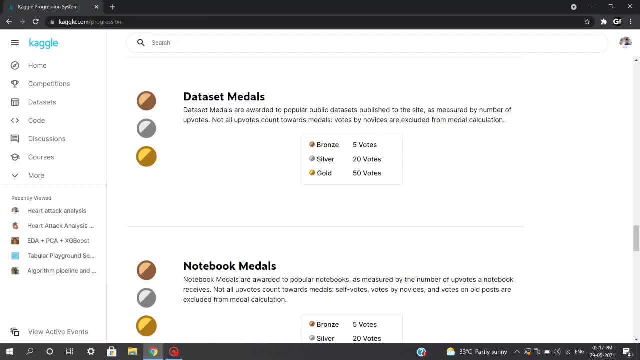 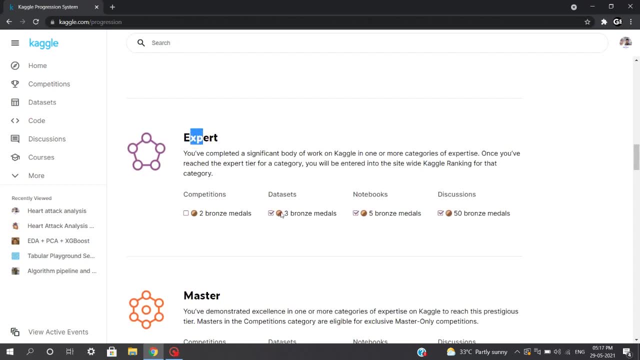 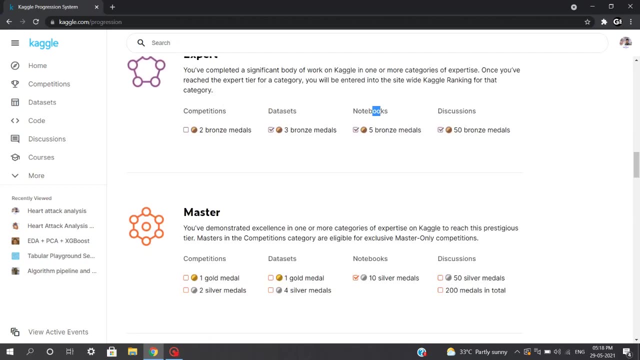 medal. if you are getting twenty upwards you will be awarded as a silver medal and if you are getting 50 upwards you will be awarded as a gold medal. and coming towards the years to get into expert here you need three bronze medals for data set and five bronze medals for notebooks. for coming to 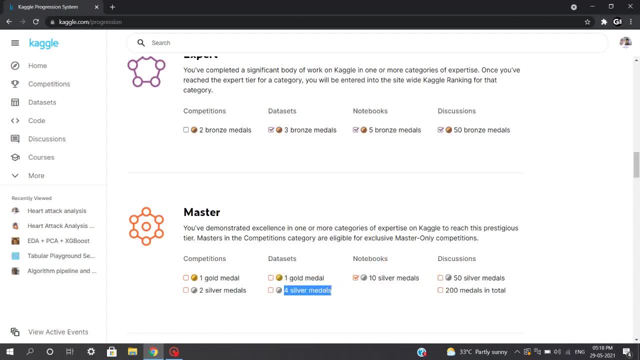 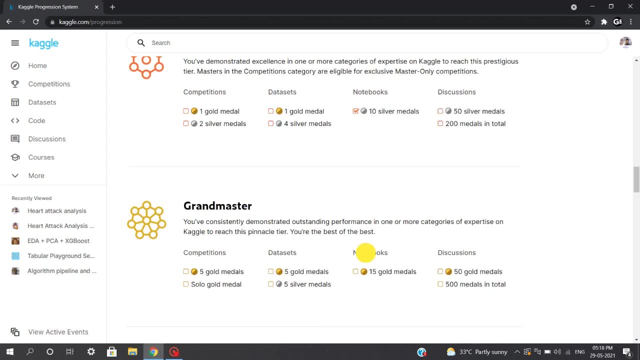 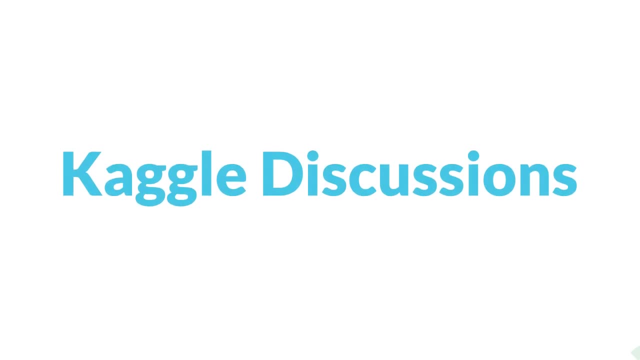 master, you need ten silver medals, for four silver medals for master and for the prestigious grand master rank, you need 15 gold medals for notebook, while five gold medals and five silver medals for data sets. Now, coming towards the discussion section, this is the best part of the Kaggle which I admire the most. 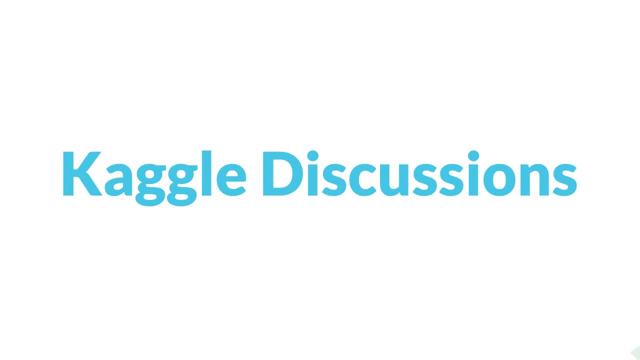 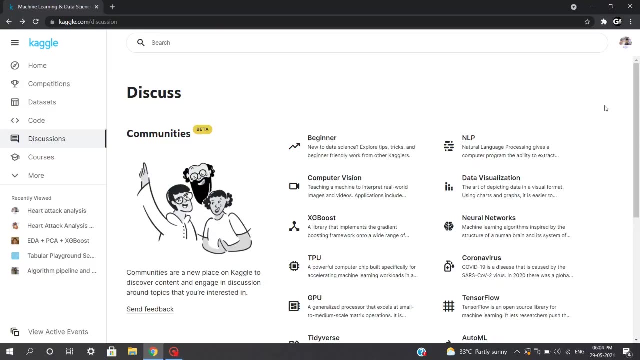 like Medium, GitHub, Stack Overflow and LinkedIn, Kaggle serves a huge community where data analysts, data scientists, machine learning engineers can come to learn, grow and network. The Kaggle discussion section is divided into various subsections, such as Beginner, NLP, Data Visualization. 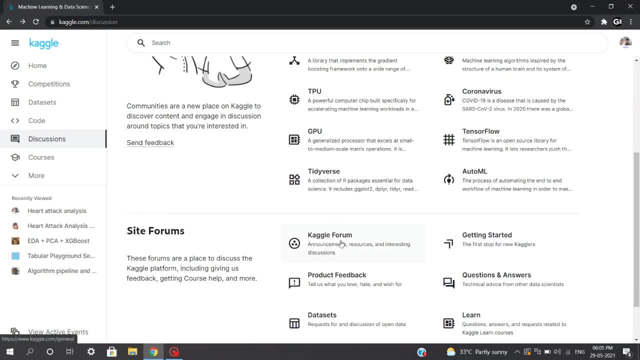 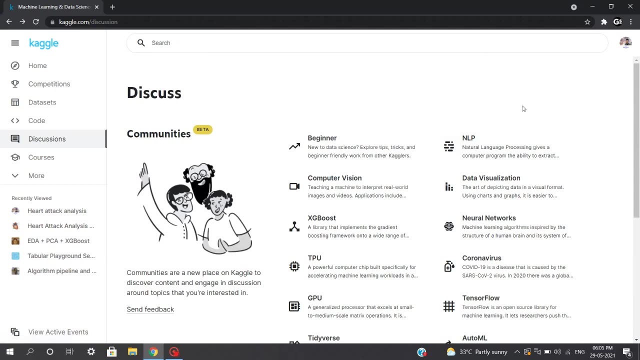 ExeBoost, and there are also site forums such as Kaggle Forum, Getting Started- Question Answers. So Getting Started is basically a first job for new Kagglers, curated especially for beginners. Now, for example, you got into doubt regarding NLP, that is, Natural Language Processing, so you need 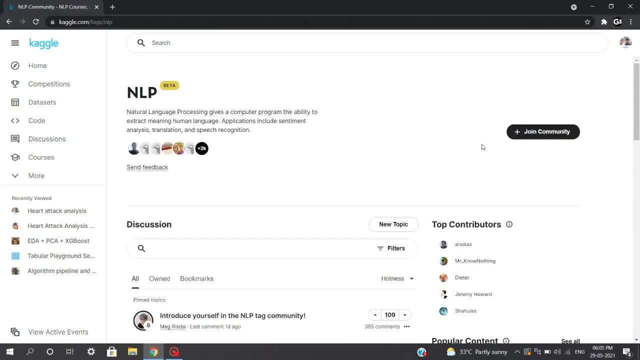 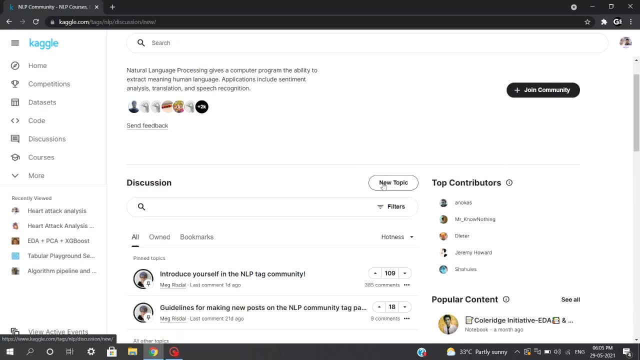 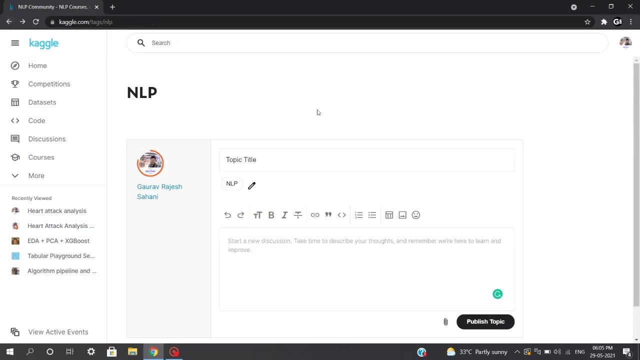 to click over here. Now you can join community to get the latest updates regarding the discussion questions and if you have the doubt, you can click on new topic. you can add the topic title and the description regarding your doubt. Now even you can contribute by solving doubts. 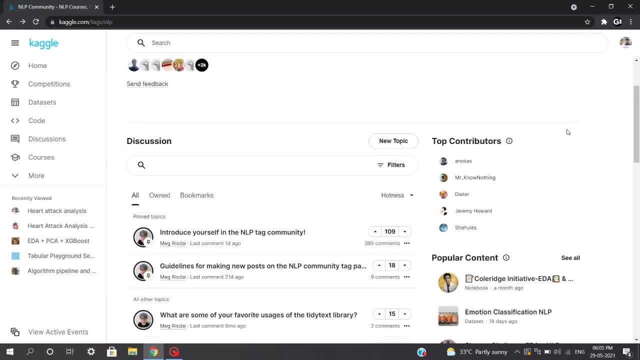 of other Kagglers and sharing some useful content to the community. After all, it is all about learning and sharing. the more you learn here, try to give back to community to grow faster, Coming towards the progression. for discussions, you just need one upload. 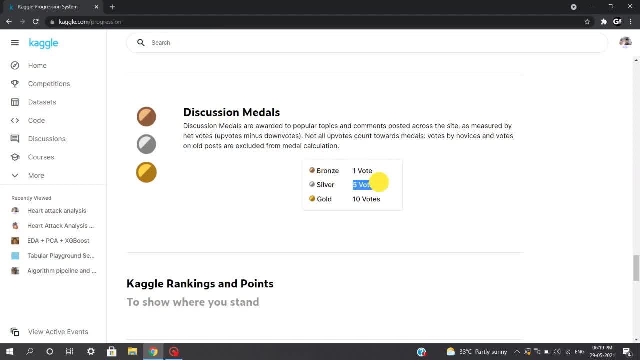 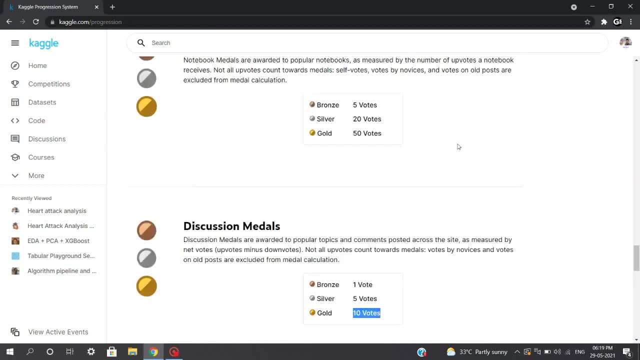 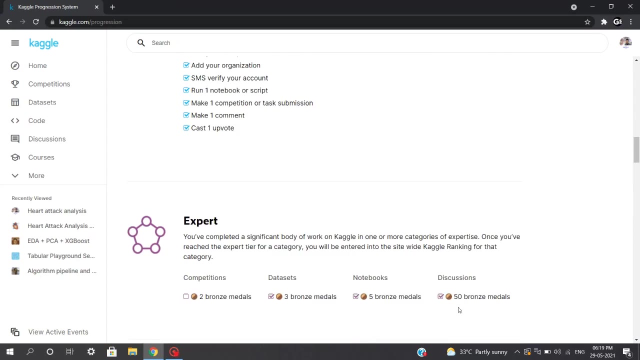 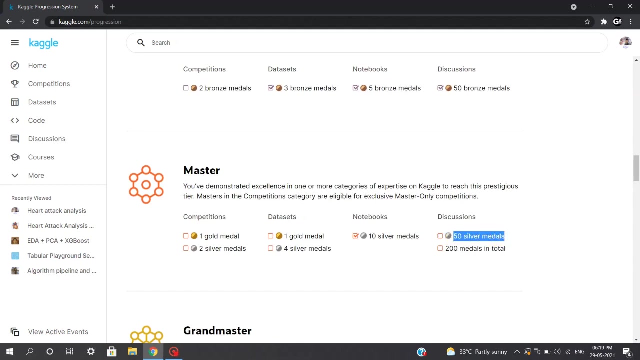 to get awarded a bronze medal, you need five reports to get awarded as a silver medal and, finally, you need ten reports to get awarded as a gold medal. now talking about the tiers for coming to expert rank, you need 50 bronze medals now from expert to master tier. you need 50 silver medals, with 200 medals in. 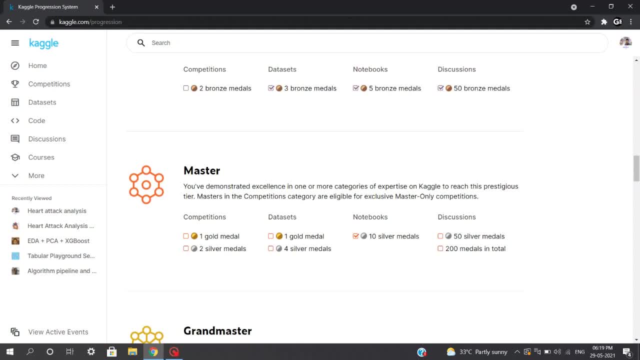 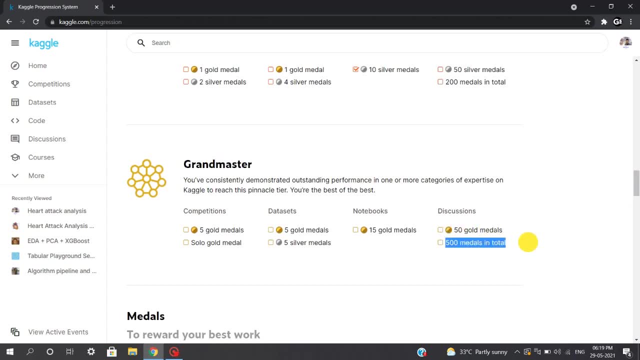 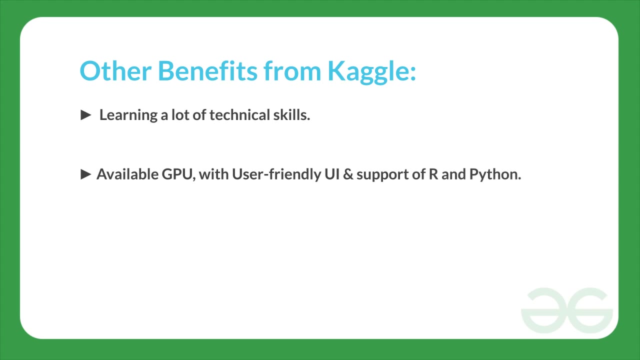 total, so this may include bronze and silver, as well as gold. now, for coming to this grand master rank, you need 50 gold medals and 500 medals in total. lastly, you can learn a lot of technical skills from here. you can learn from others work as well as you can implement by yourself. even I have learned a lot of things from